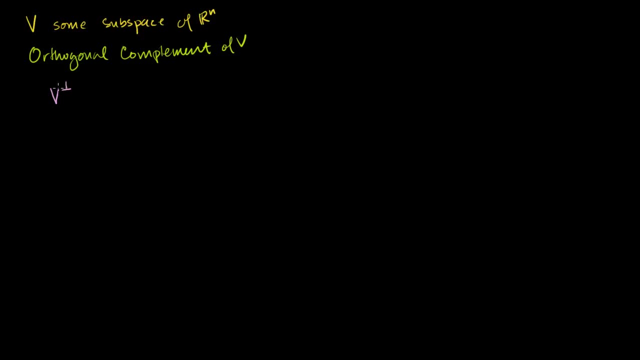 orthogonal complement of V. So we write this little orthogonal notation as a superscript on V And you can pronounce this as V perp, not for perpetrator, but more perpendicular. So V perp is equal to the set of all the vectors x that are: 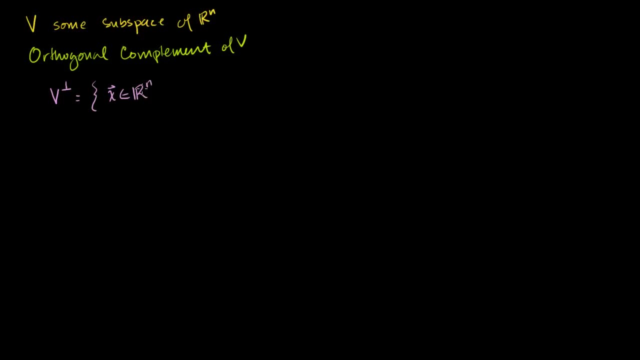 a member of our Rn, Such that x dot V is equal to 0 for every vector V that is a member of our subspace. So we're essentially saying: look, you have some subspace, It's got a bunch of vectors in it. 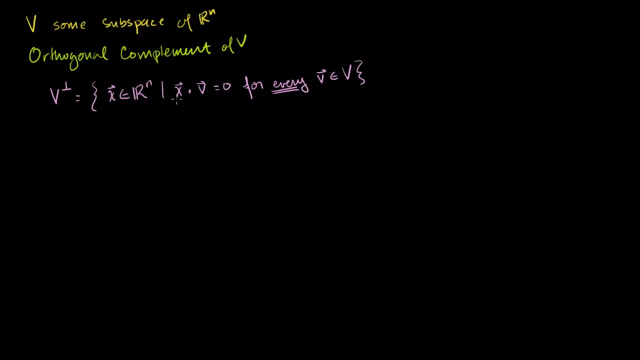 Now, if I can find some other set of vectors where every member of that set is orthogonal to every member of the subspace in question, then the set of those vectors is called the orthogonal complement of V, And you write it this way: V perp, right there. 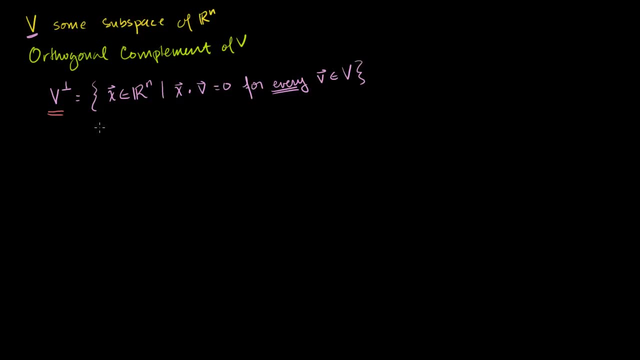 So the first thing that we just tend to do when we're defining a space or defining some set is to see: hey, is this a subspace? Is V perp or is the orthogonal complement of V? is this a subspace? 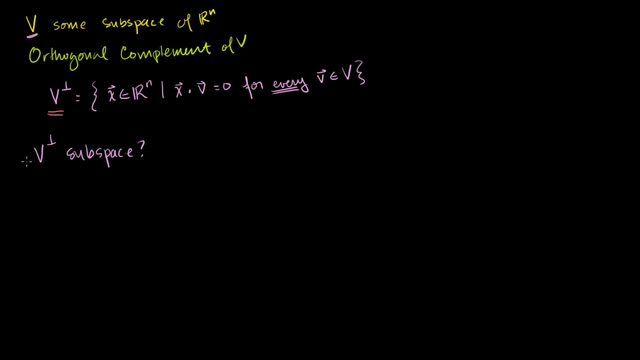 Well, you might remember from many, many videos ago that we had just a couple of conditions for a subspace, That if let's say that a and b are both a member of V perp, then we have to wonder whether a plus b is a member of V perp. 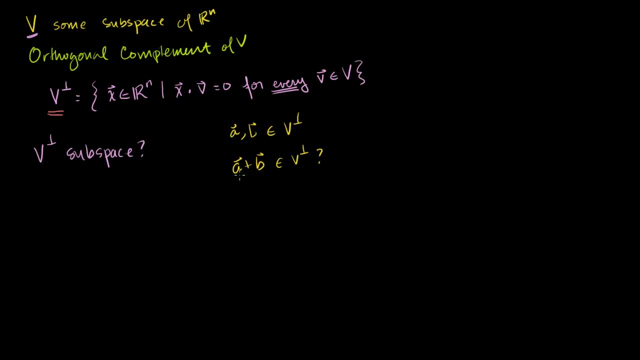 That's our first condition. It needs to be closed under addition, in order for this to be a subspace. And then the next condition is: well, if a is a member of V perp, is some scalar multiplication, So a multiple of a also a member of V perp? 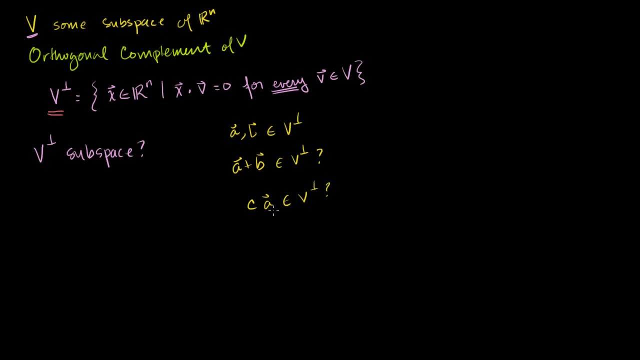 And then the last one: it has to contain the 0 vector, which is a little bit redundant with this, Because if any scalar multiple of a is a member of our orthogonal complement of V, then you can just multiply it by 0.. 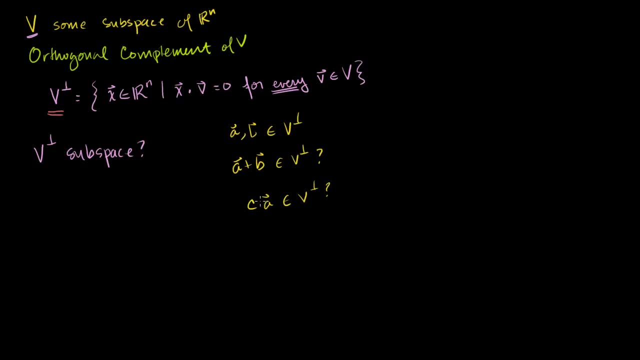 So it would imply that the 0 vector is a member of V. So what does this imply? What is the fact that a and b are a? They are members of V. perp, That means that a dot v where this v is any member of our. 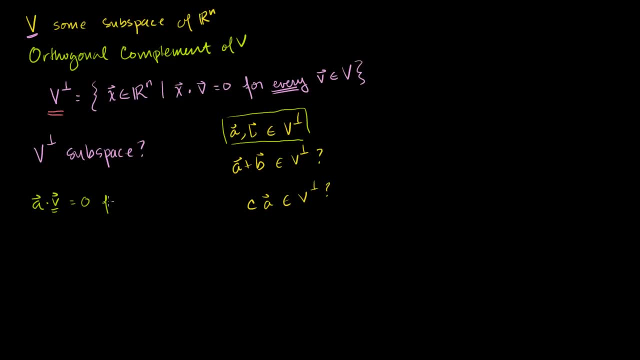 original subspace v is equal to 0 for any v that is a member of our subspace v, And it also means that b, since b is also a member of V perp, that v dot- any member of our subspace- is also going to be 0. 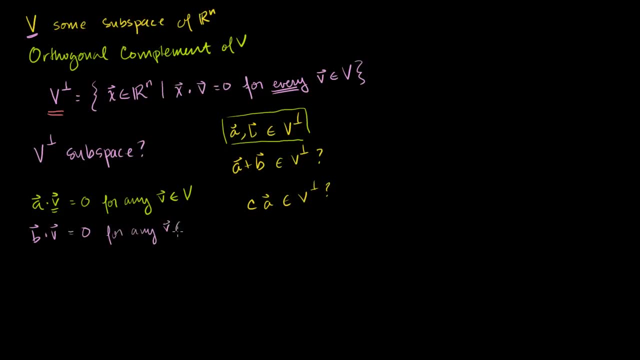 for any v That is a member of V. So what happens if we take a plus b dot v? Let's do that. So if I do a plus b dot v, what is this going to be equal to? This is going to be equal to a dot v plus b dot v. 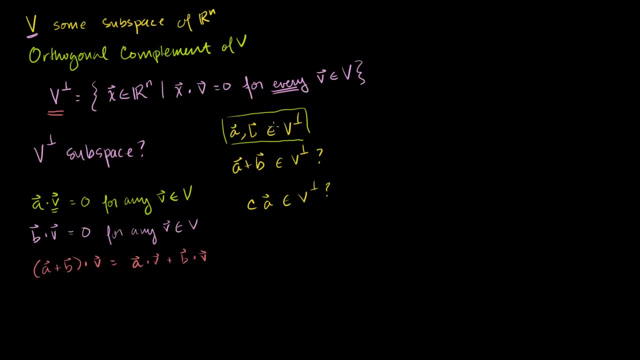 And we just said. the fact that both a and b are members of our orthogonal complement means that both of these quantities are going to be equal to 0. So this is going to be equal to 0. This is going to be equal to 0 plus 0, which is equal to 0. 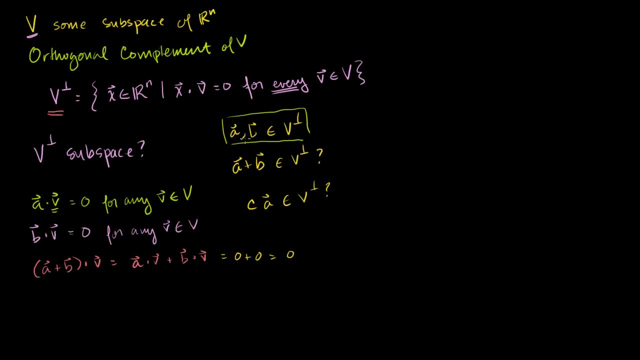 So a plus b is definitely a member of our orthogonal complement. So we've got our checkbox right there. I'll do it in a different color than the question mark. Check for the first condition for being a subspace Now is c a a member of V perp. 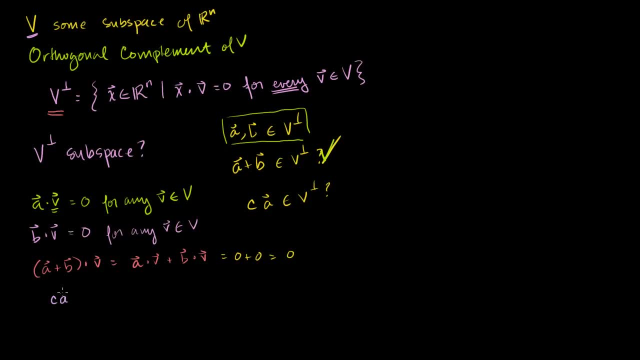 Well, let's just take c. If we take c, a and dot it with any member of our original subspace, Any member of our original subspace, This is the same thing as c times a dot v. And what is this equal to? 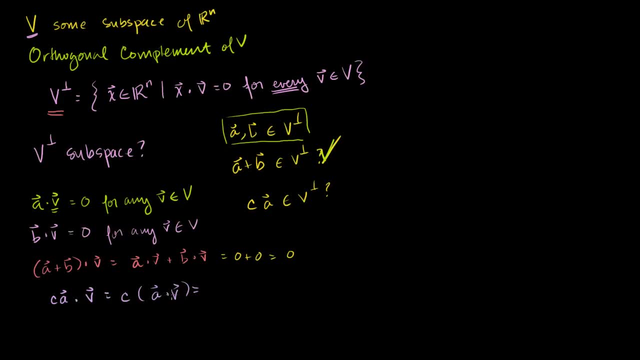 By definition, a was a member of our orthogonal complement, so this is going to be equal to 0.. So this is going to be c times 0, which is equal to 0. So this is also a member of our orthogonal complement to v. 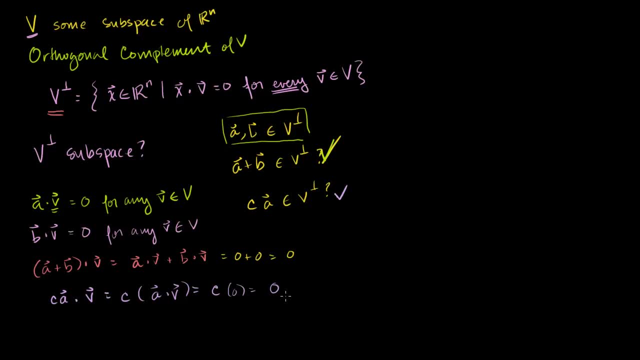 And of course I could multiply c times 0 and I would get to 0.. Or you could just say: look, 0 is orthogonal to everything. You take the 0 vector and dot it with anything, you're going 0,. so the 0 vector is always going to be a member of any. 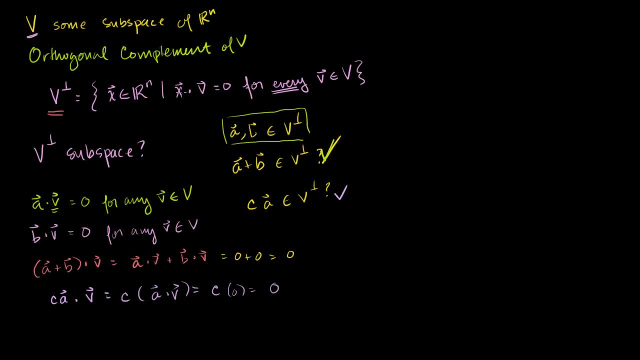 orthogonal complement, because it obviously is always going to be true for this condition right here. So we know that v, perp, or the orthogonal complement of v, is a subspace, which is nice, because now we can apply to it all of the properties that we know of subspaces. 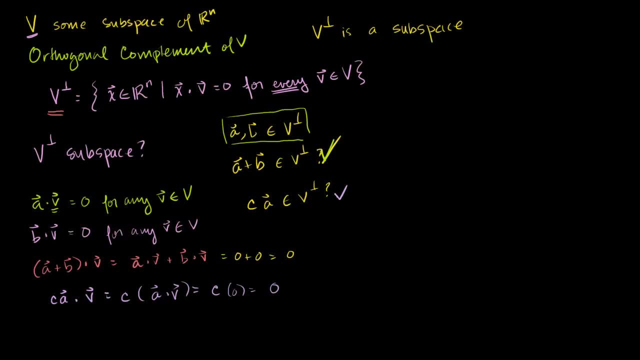 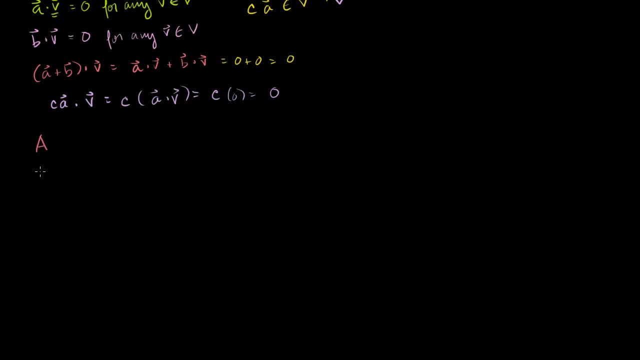 Now the next question, and I touched on this in the last video. I kind of just touched on the idea. I said that if I have some matrix A and let's just say it's an m by n matrix- In the last video I said that the row space of A is well 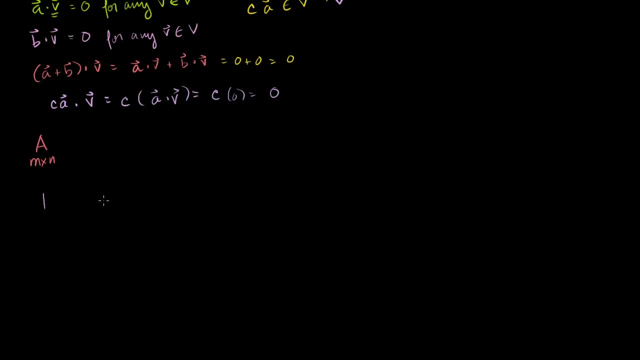 let me write it this way. I wrote that the null space of A- let me switch this up the order- the null space of A is equal to the orthogonal complement of the row space of A And in a way that we can write the row space of A this thing: 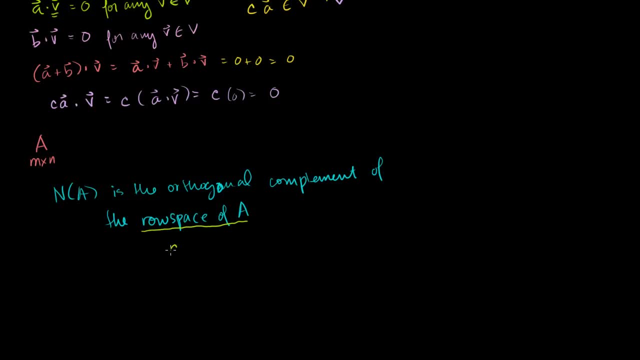 right here. the row space of A is the same thing as the column space of A transpose. So one way you could rewrite this sentence right here is that the null space of A is the orthogonal complement of the row space. The row space is the column space of the transpose matrix. 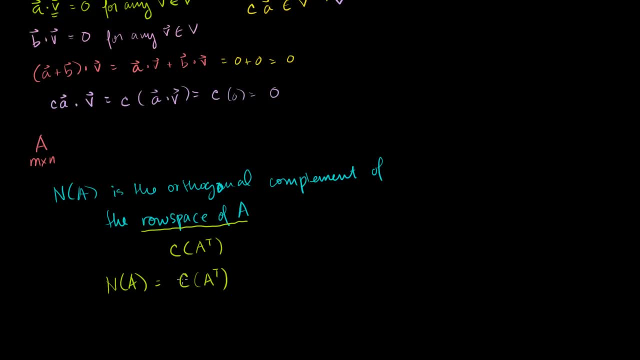 And the claim, which I have not proven to you, is that this is the orthogonal complement of this, So this is equal to that, The little perpendicular superscript. That's the claim, And at least in the particular example that I did in the last. 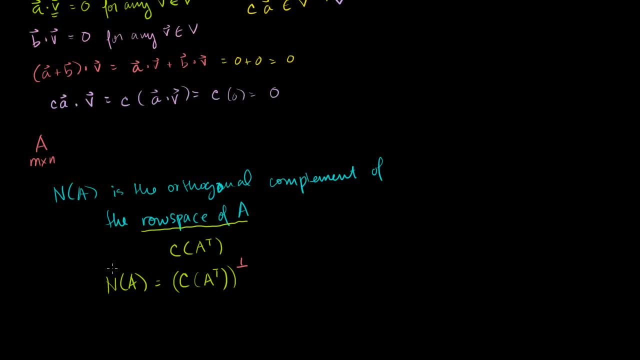 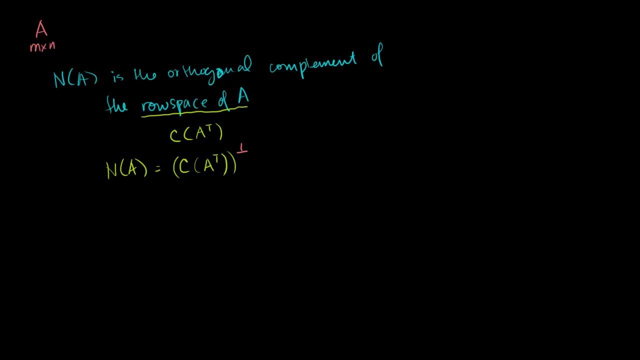 two videos. this was the case where I actually showed you that 2 by 3 matrix, But let's see if this applies generally. So let me write my matrix A like this. So my matrix A, I can write it as just a bunch of row vectors. 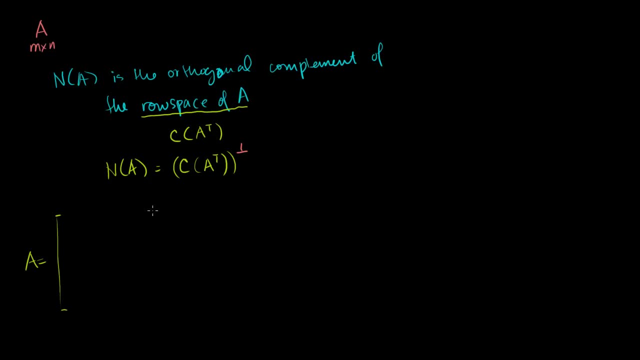 But just to be consistent with our notation, well, vectors we tend to associate as column vectors. So to represent the row vectors here, I'm just going to write them as transpose vectors, Because in our reality vectors will always be column vectors. 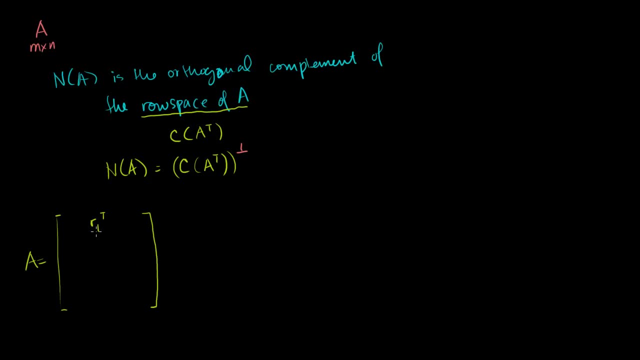 and row vectors are just transposes of those: R1 transpose, R2 transpose and you go all the way down. We have m rows, So you're going to get Rm transpose. Don't let the transpose part confuse you. I'm just saying that these are row vectors. 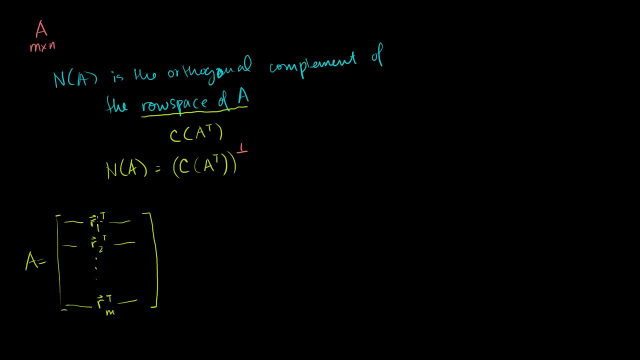 I'm writing transposes there just to say that, look, these are the transposes of column vectors that represent these rows. But if it's helpful for you to imagine them, just imagine: this is the first row of the matrix. This is the second row of that matrix. 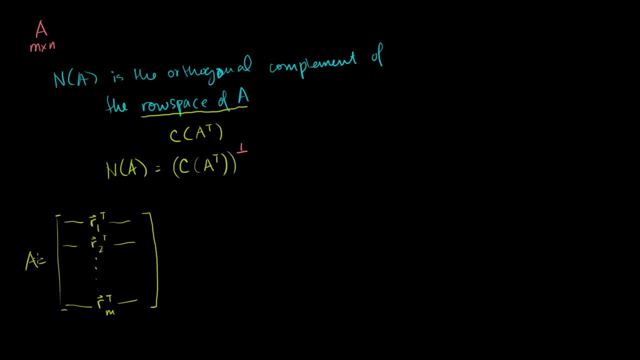 So on and so forth. Now, what is the null space of A? Well, that's all of the vectors here. Let me do it like this: The null space of A, Let me write it like this: It's all of the vectors x that satisfy the equation that this. 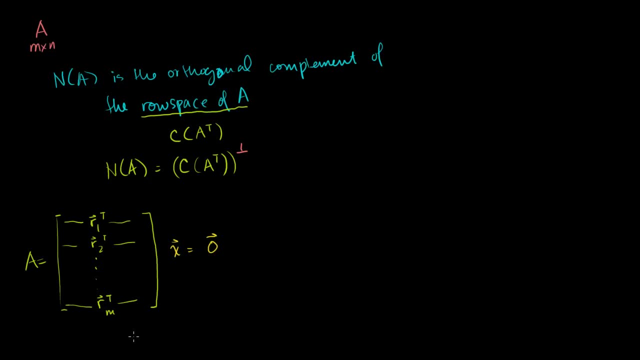 is going to be equal to the 0 vector. Now, to solve this equation, what can we do? We've seen this multiple times. This matrix vector product is essentially the same thing as saying: let me write it like this a little bit: 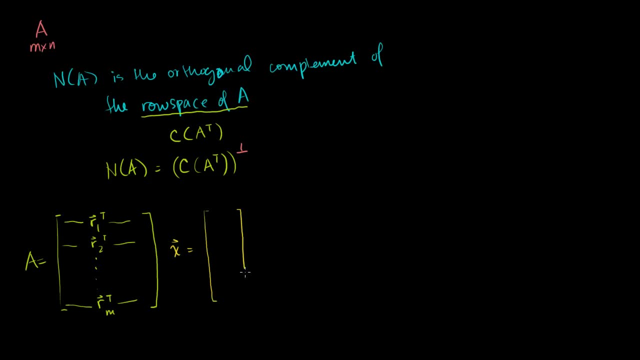 Let me write it like this: It's going to be equal to the 0 vector in Rm, So you're going to have m zeros. It's going to go all the way down to the mth of 0.. So another way to write this equation. you've seen it before. 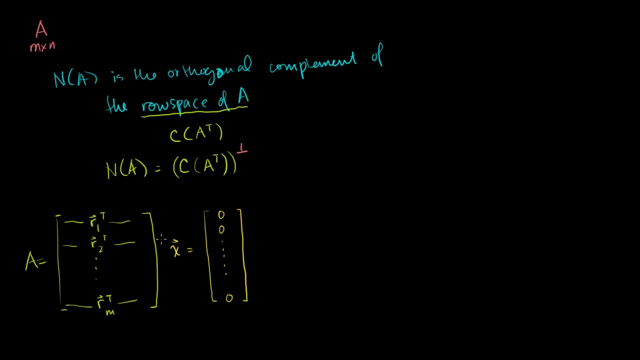 is when you take the matrix vector product, you're essentially taking the dot product. So to get to this entry right here, this entry right here is going to be this row dotted with my vector x, So this is R1.. We're calling this row vector R1. transpose. 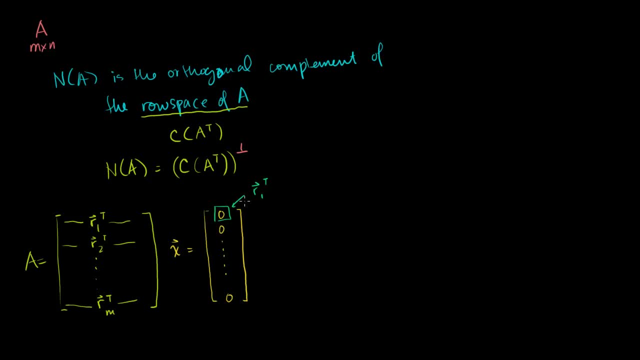 It's the transpose of some column vector that can represent that row, But that dot, dot, my vector x, this vector x is going to be equal to that 0.. Now, if I take this guy, let me do it in a different color. 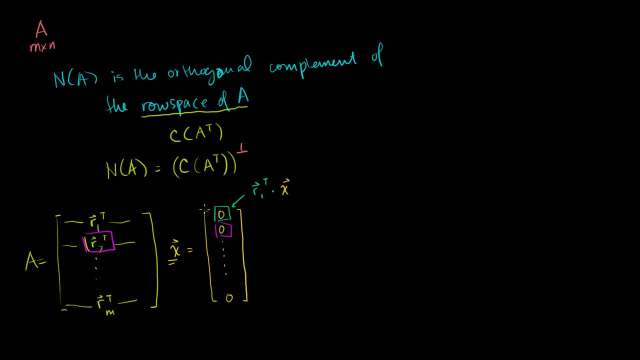 If I take this guy and I dot him with vector x, it's going to be equal to that 0. So R2 transpose dot x is going to be equal to that 0, right there. So by definition, or I guess let me write it this way: 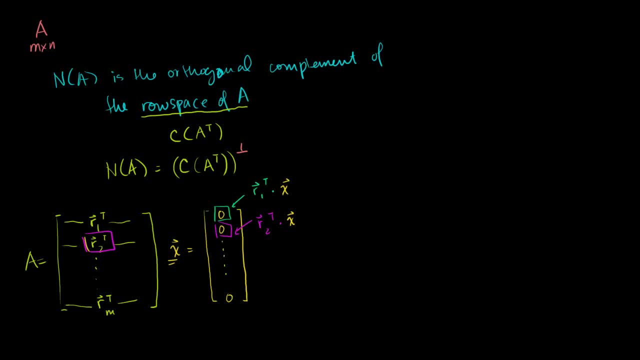 Another way to write this equation is to write it like this: R1- transpose dot x, is equal to 0,. R2, transpose dot x, is equal to 0,. all the way down to Rn- transpose dot x is equal to 0.. 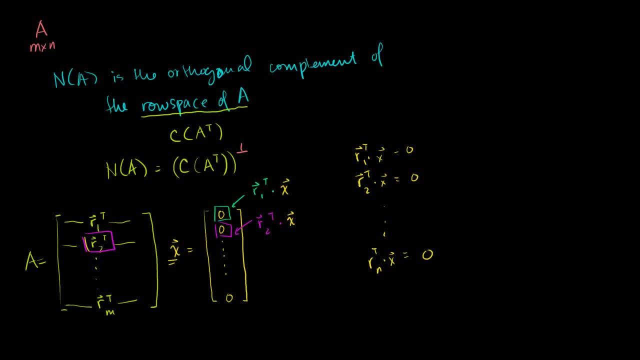 And, by definition, the null space of A. the null space of A is equal to all of the x's that are members of- in this case it's an m by n matrix, so you're going to have n columns, So it's all the x's that are members of Rn, such that Ax is. 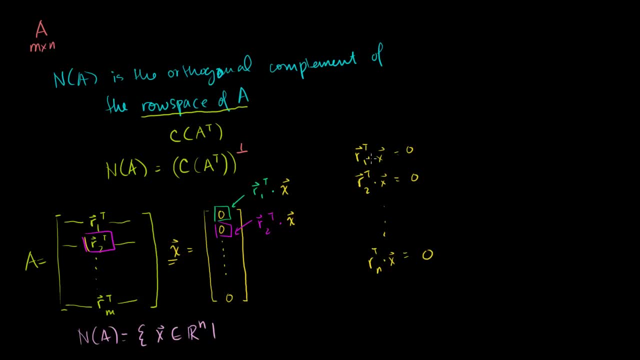 equal to 0.. Or you could alternatively write it this way that if you were to dot each of the rows with x, you're going to be equal to 0. So you could write it this way. Well, let me just write it such that Ax is equal to 0.. 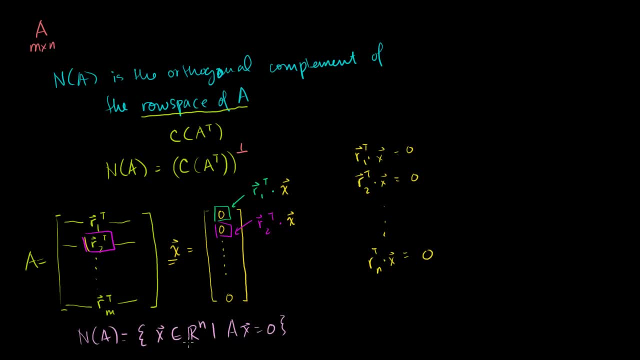 So you could write it this way. You could well let me just write it such that Ax is equal to 0. That's an easier way to write it. So let's think about it. If someone is a member, if, by definition, I give you some. 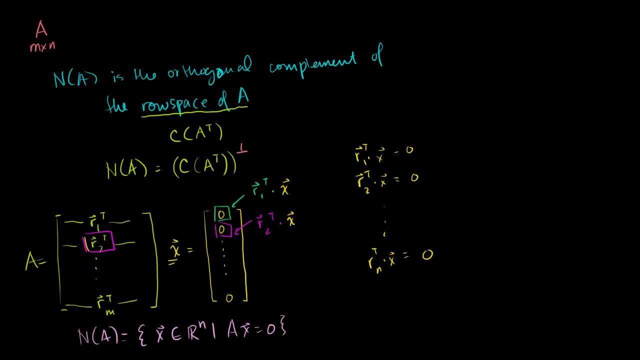 vector v. if I say that, let me switch colors. if I were to tell you that v is a member of the null space of A, I just tell you: let's call it v1.. v1 is a member of null space of A. 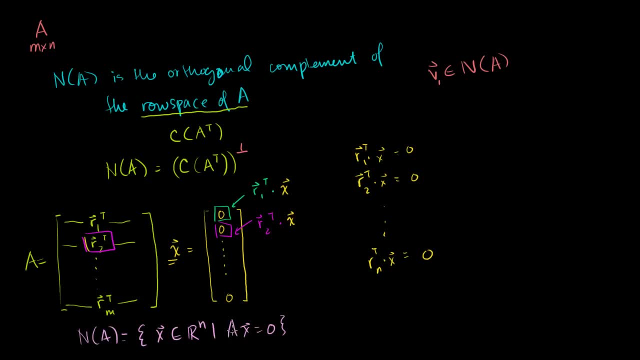 That means it satisfies this equation right here. That means A times v is equal to 0.. A times v is equal to 0 means that when you dot each of these rows with v, you get equal to 0.. Or another way of saying that is that v1 is orthogonal to. 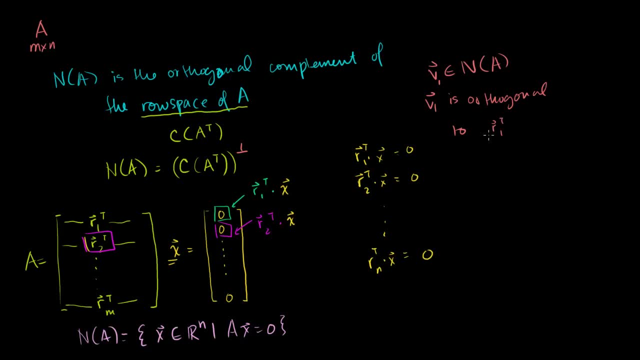 all of these rows To R1 transpose. that's just the first row. R2 transpose all the way to Rm. All the way to Rm transpose. All the way to Rm transpose. So this is orthogonal to all of these guys by definition. 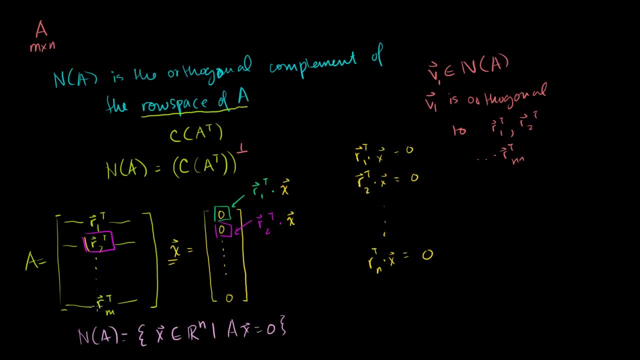 any member of the null space. Well, if you're orthogonal to all of these rows in your matrix, you're also orthogonal to any linear combination of them. You're also orthogonal to any linear combination, Orthogonal to any linear combination, And you can imagine, let's say that we have some vector, that 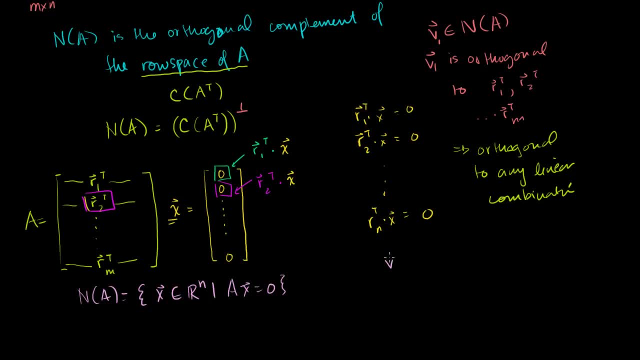 is a linear combination of these guys right here. So let's say vector. let me write it well, it's going to be a member of the R space. Let me think of a good. I want to do it different. Let's say vector w is equal to some linear combination of. 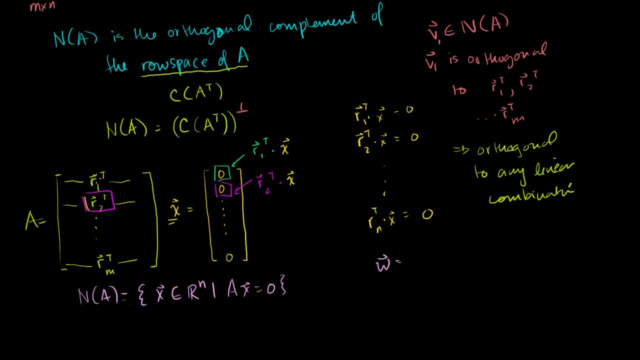 these vectors right here. I wrote them as transposes just because they're row vectors, but I could just write them as regular vectors, Regular column vectors, just to show that w could be just a regular column vector. So let's say w is equal to c1 times R1 plus c2 times R2, all. 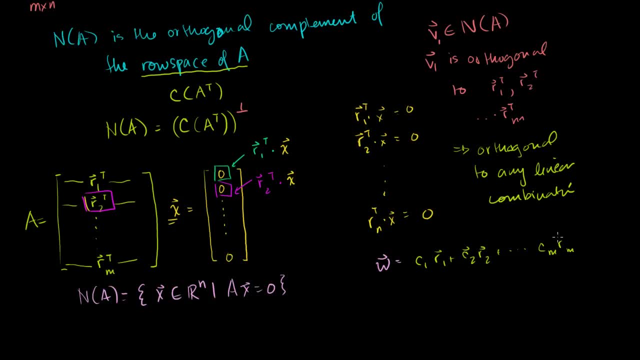 the way to cm times Rm. That's what w is equal to. So what happens when you take v, which is a member of our null space, and you dot it with w? So if we were to take v and dot it with w, it's going to be. 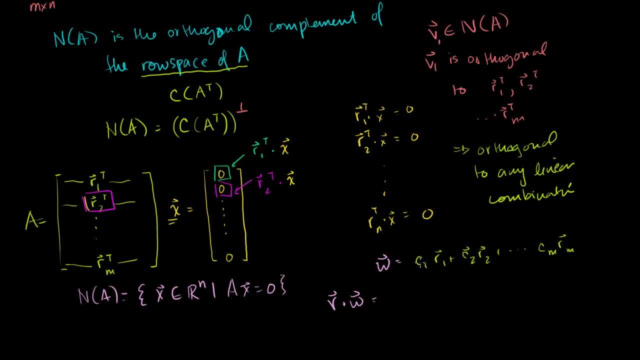 v dot with each of these guys, because our dot product has the distributive property. So if you dot v with each of these guys it's going to be equal to c1, I'm just going to take the scalar out: c1 times. 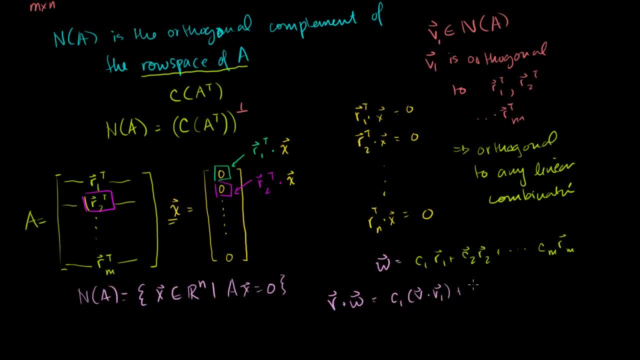 v dot R1 plus c2 times v v dot R2.. This is an R right here, not a v Plus all the way to plus cm times v dot rm. And we know we already just said that v dot each of these. 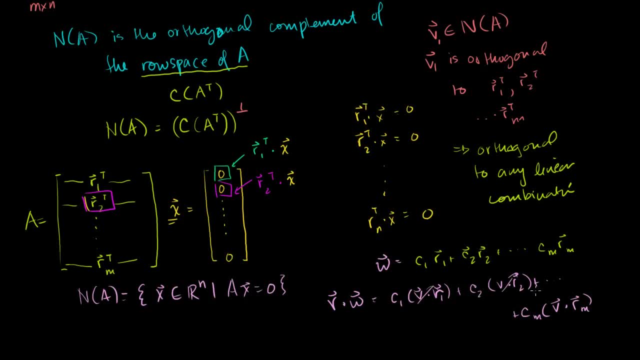 r's are going to be equal to 0. So all of these are going to be equal to 0. So this whole expression is going to be equal to 0.. So if you have any vector, that's a linear combination of these row vectors. if you dot it with any member of your 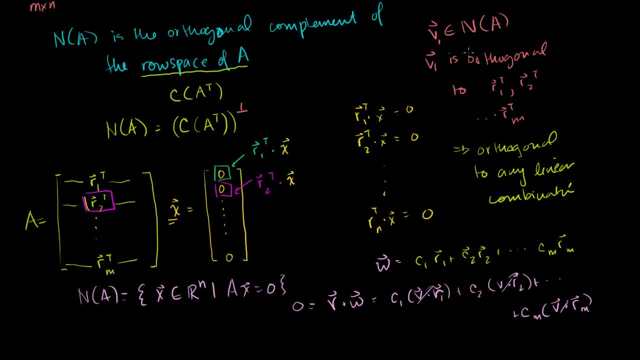 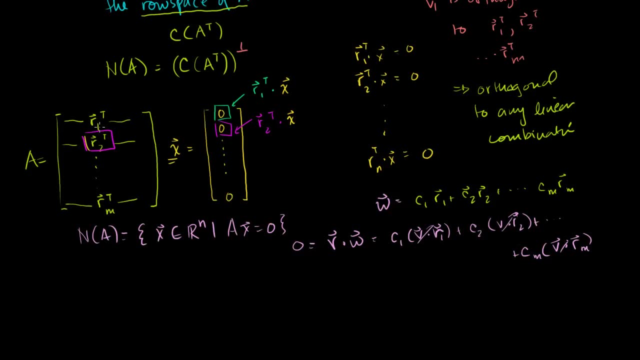 null space, you're going to get 0.. So let me write it this way: What is any vector, that's any linear combination of these guys? Well, that's the span of these guys, Or you could say that the row space. 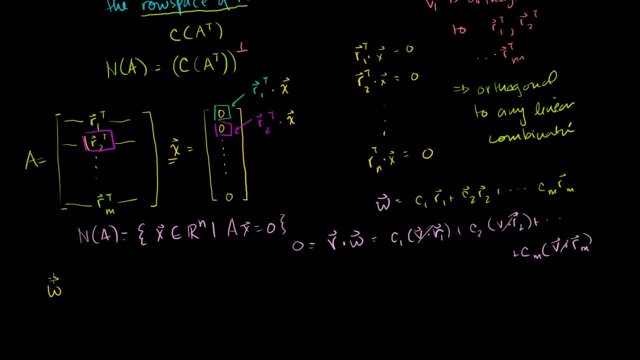 That's the row space. So if w is a member of the row space which you can just represent as a column space of a transpose, then we know, and let's say we know- that v is a member of our null space. we. 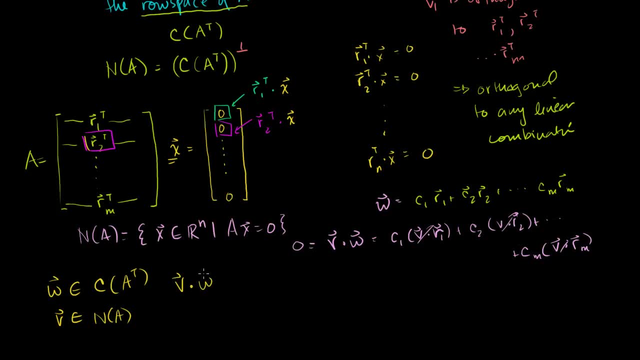 know that v dot w is going to be equal to 0.. I just showed that to you right there. So every member of our null space is definitely orthogonal to every member of our row space. So that's what we know so far. Every member of null space of A is orthogonal to every 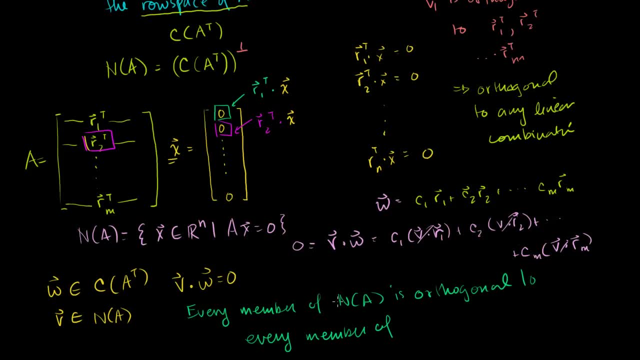 member of the row space. So if w is to the row space of A now, that only gives us halfway. That still doesn't tell us that this is equivalent to the orthogonal complement of the null space. For example, there might be members of our orthogonal 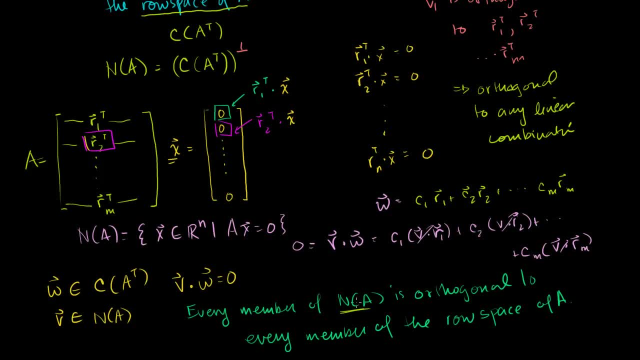 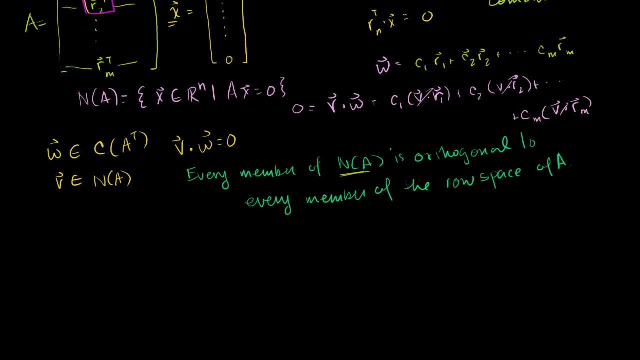 complement of the row space that aren't a member of our null space. So let's say that I have some other vector That is. let's say I have some vector u. Let's say that u is A member- is a member of the orthogonal complement of our row space. 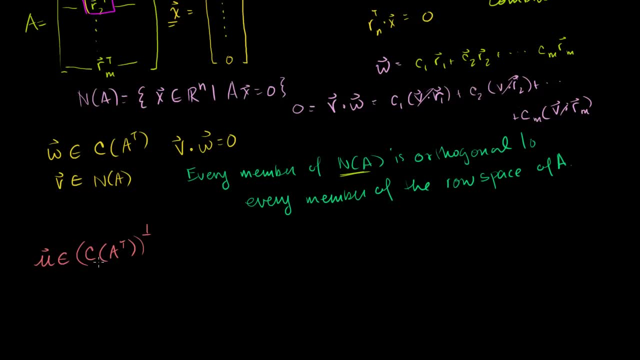 I know the notation is a little convoluted. Maybe I should write an r there. But I want to really get set in your mind that the row space is just the column space of the transpose. So let's say that u is some member of our orthogonal complement. 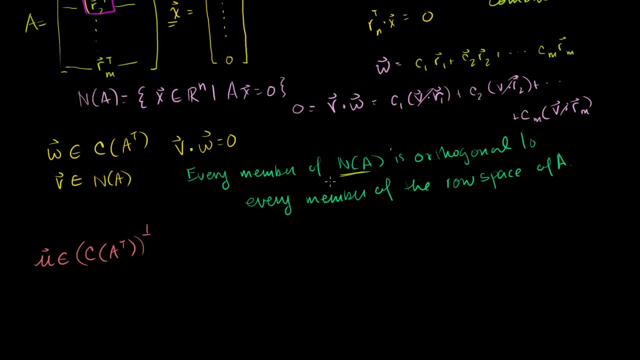 What I want to do is show you that u has to be in your null space. When I show you that, then we know So far, we just said that OK, Then everything OK. in the null space is orthogonal to the row space. 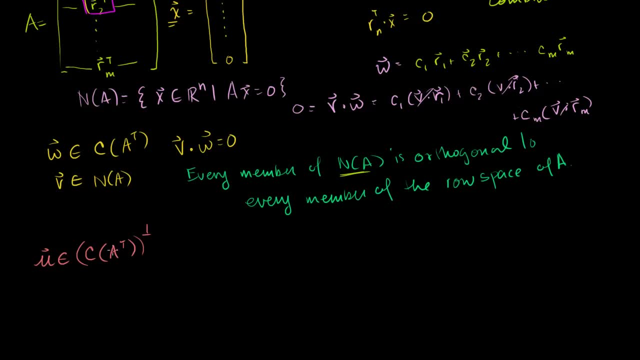 But we don't know that everything that's orthogonal to the row space which is represented by this set is also going to be in your null space. That's what we have to show in order for those two sets to be equivalent, in order for the null space to be equal to this. 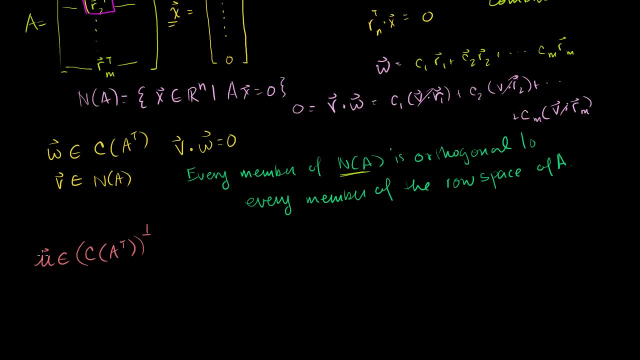 So if we know this is true, then this means that u dot w where w is a member of our row, space is going to be equal to 0.. It's going to be equal to 0.. Let me write this down right here. 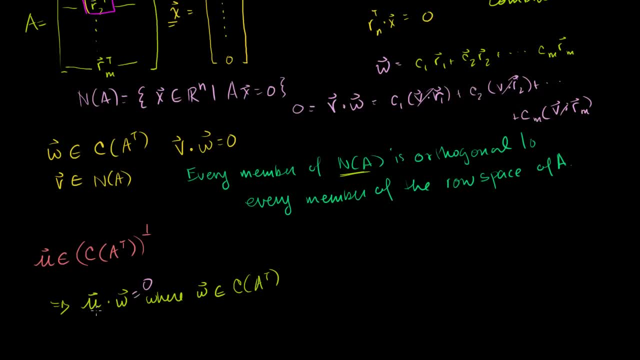 That is going to be equal to 0.. And what does that mean? That means that u is also orthogonal. so this implies that u, dot w is also orthogonal. Well, rj- any of the row vectors- is also equal to 0,. 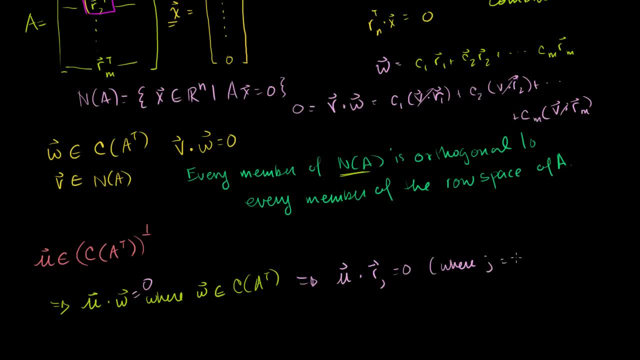 where j is equal to 1 all the way through m. How do I know that? Well, I'm saying that. look. u is a member of the orthogonal complement of the row space. So that means u is orthogonal to any member of your row. 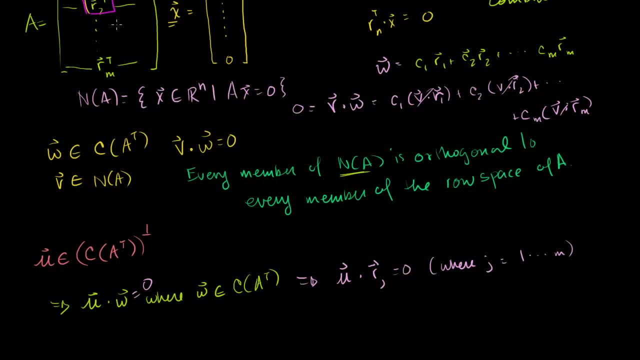 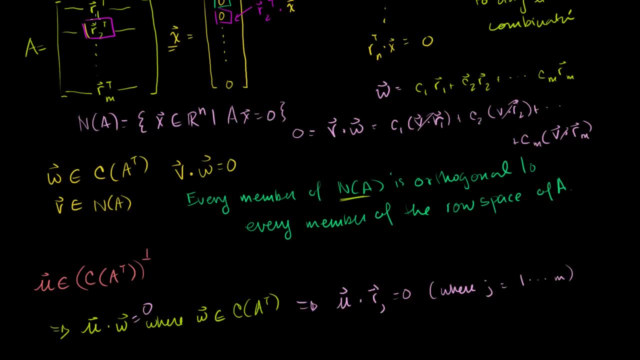 space, so, in particular, the basis vectors of your row space. we don't know whether all of these guys are basis vectors, But that means we can take. these guys are definitely all members of the row space. Some of them are actually the basis for the row space. 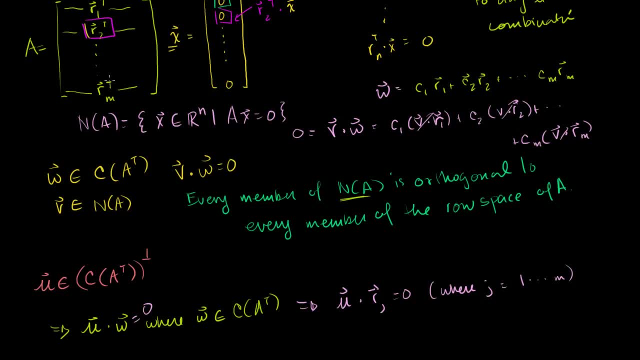 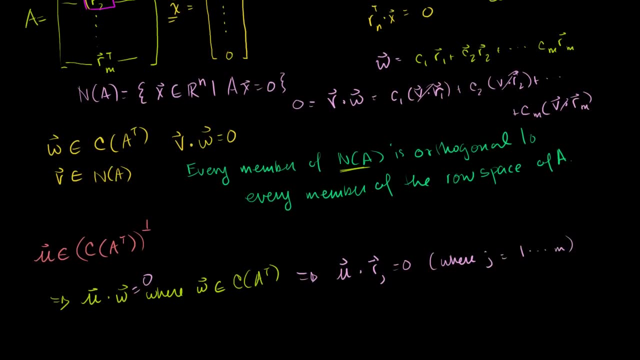 So that means if you take u dot in any of these guys, it's going to be equal to 0. So if u dot any of these guys is equal to 0, that means that u dot r1 is 0.. Let me write this down. 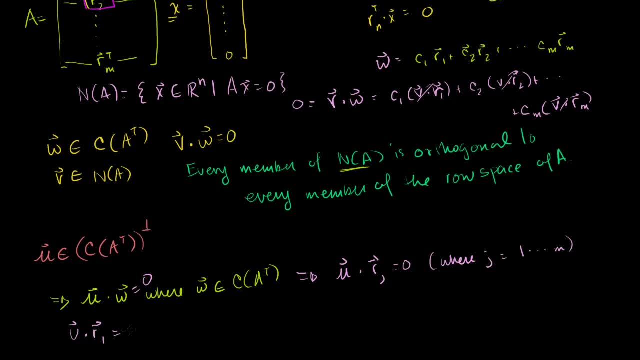 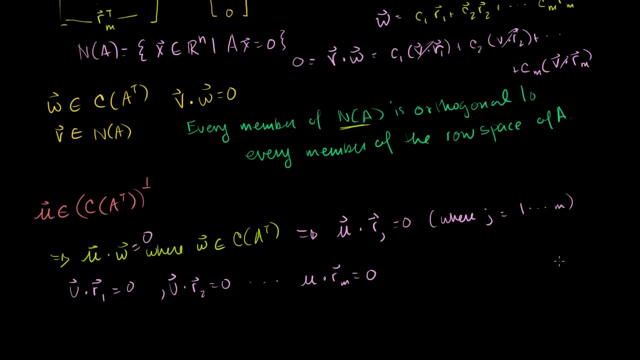 u dot r1 is equal to 0.. u dot r2 is equal to 0.. All the way to: u? u dot rm is equal to 0.. Well, if all of this is true, that means that a times the vector u is equal to 0. 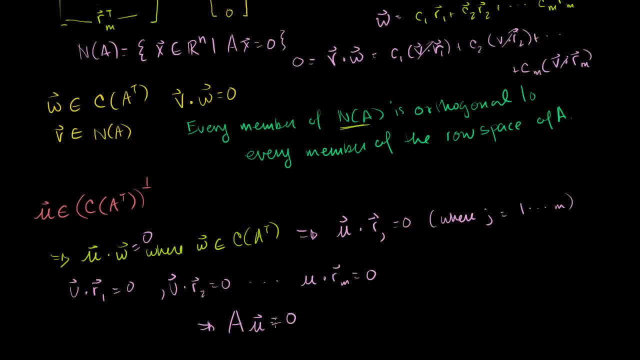 That implies this: right, You stick u there, you take all the dot products. it's going to satisfy this equation, which implies that u is a member of our null space. So we've just shown you that every member of your null space is definitely a member of the orthogonal complement. 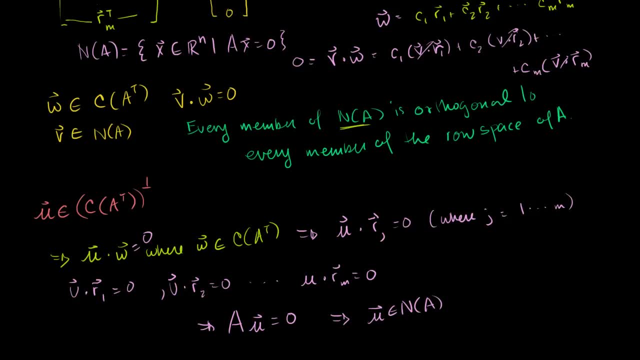 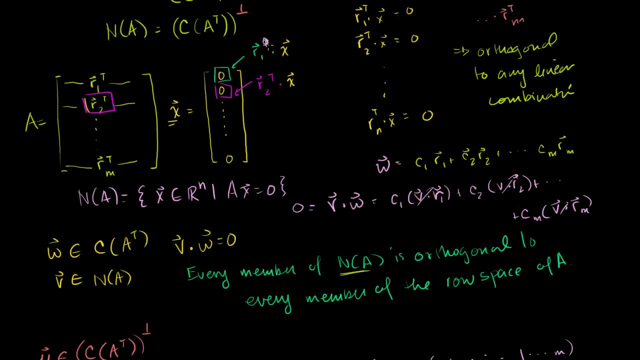 And now we said that every member of our orthogonal complement is a member of our null space, Is a member of our null space. And actually I just noticed that I made a slight error here. This dot product. I don't have to write the transpose here. 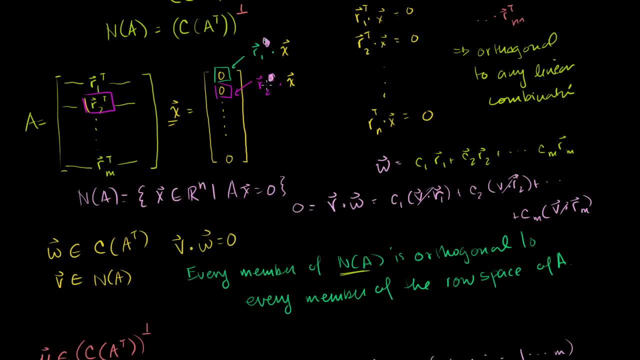 because we've defined our dot product as the dot product of column vectors. So this is the transpose of some column vector. So you can untranspose it here and just take the dot product. But anyway, minor error there. But that diverts me from my main takeaway, my punch line. 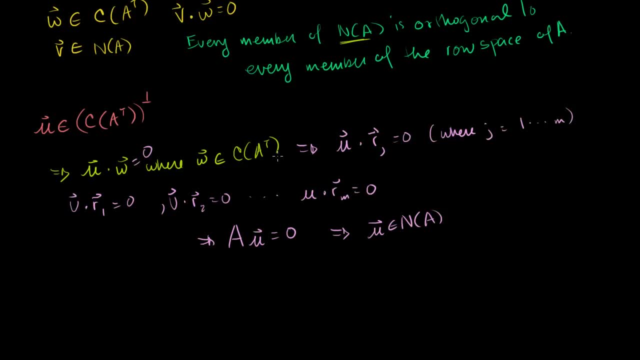 the big picture We now showed you. any member of our null space is a member of the orthogonal complement. So we just showed you this first statement. here is another way of saying any member of the null space, or that the null space is a subset of the orthogonal complement of the. 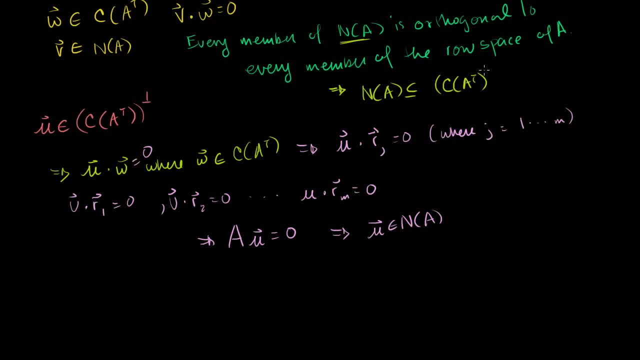 row space. So that's our row space and that's the orthogonal complement of our row space. And here we just showed that any member of the orthogonal complement of our row space is also a member of your null space. Well, if these two guys are subsets, then we're going to be. 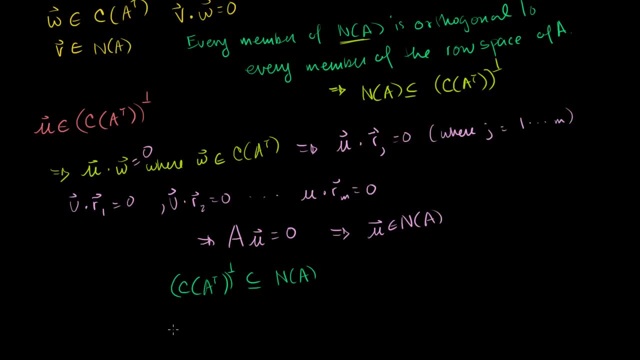 able to show that they must be equal to each other. So we now know that the null space of A is equal to the orthogonal complement of the row space of A, or the column space of A. transpose Now this is: I related the null space with the row space. 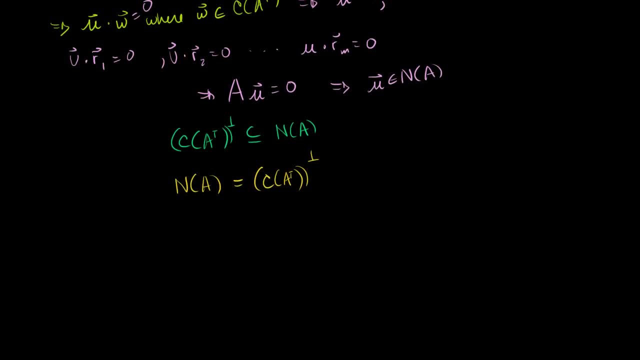 Now I could just as easily make a bit of a substitution here. Let's say that A is equal to some other set of sets, Let's do that. Let's say A is equal to some other set of sets, Let's do that. 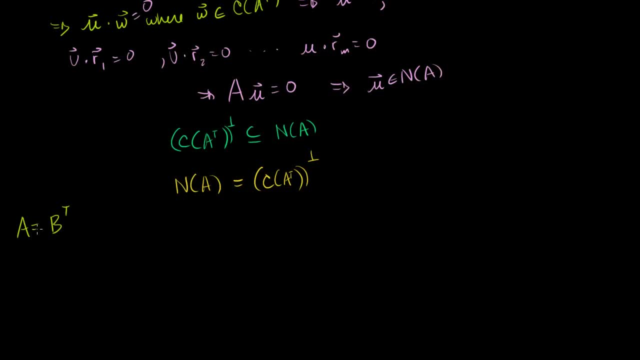 other matrix, B transpose. right, It's going to be the transpose of some matrix You could transpose either way. So if I just make that substitution here, what do we get? We get: the null space of B transpose is equal to the column space of. let me write it out: B transpose, transpose. 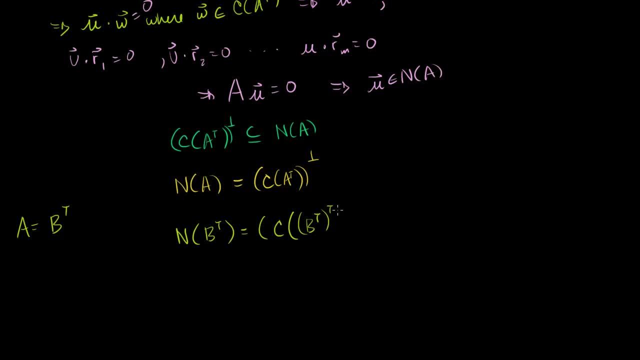 right. A transpose is B transpose transposed. Let me get my parentheses right. And then that thing's orthogonal complement. So what is this equal to This? the transpose of the transpose is just equal to B, So I could write it as the null space of B transpose is. 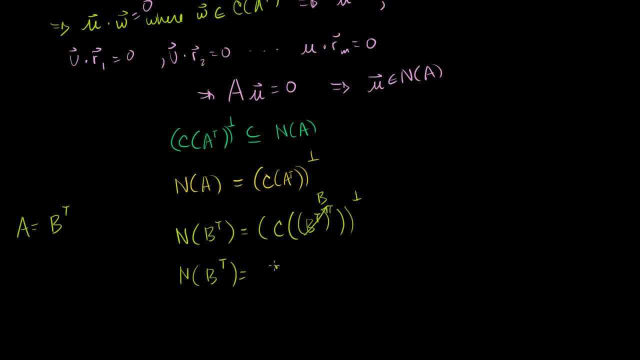 equal to the orthogonal complement of the column space of B, the orthogonal complement of the column space of B. So, just like this, we just showed that the left, you know B and A, they're just arbitrary matrices. So this showed us that the null space, so this is null.